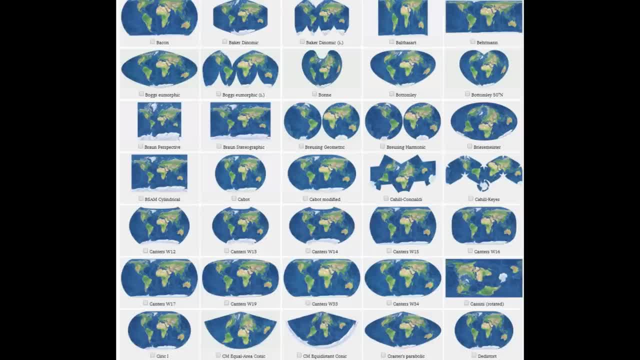 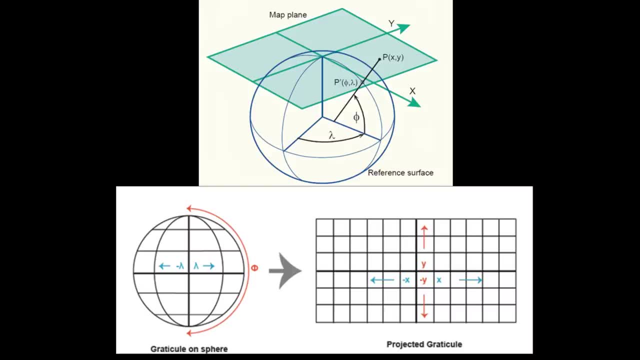 all of them. So essentially a map projection is a cartographer's take on those compromises and it's all based on math and geometry and it can get pretty complicated as well. I'm not going to get into the math of it all because I can't, but because it is math, there are essentially an infinite number of map. 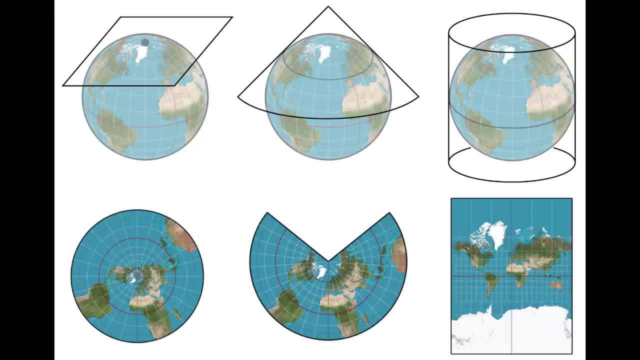 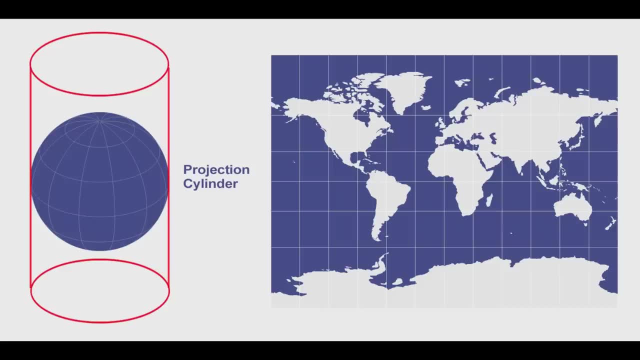 projections possible. For getting the actual image onto a piece of paper. the three major methods are cylindrical, conical and planar. For a cylindrical projection, imagine a piece of paper being wrapped around the globe like a cylinder. So if it's light the map is projected. but as it's rolled out you can see how the polar areas are going to be stretched. 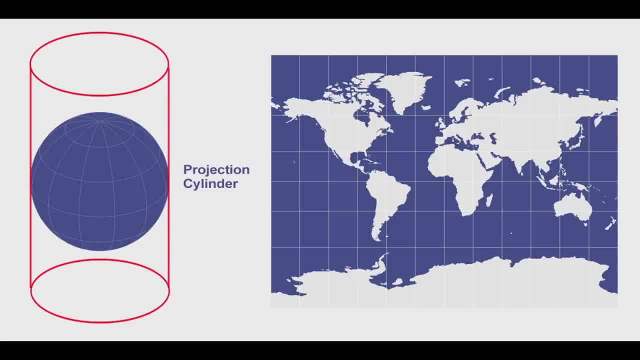 And there's not one type of cylindrical projection. there are many that are based off of this. So by messing around with the math you can make the maps look a lot different, even though you're still using a cylindrical projection For a conical map. imagine placing a cone-shaped piece of paper on the globe like a hat. 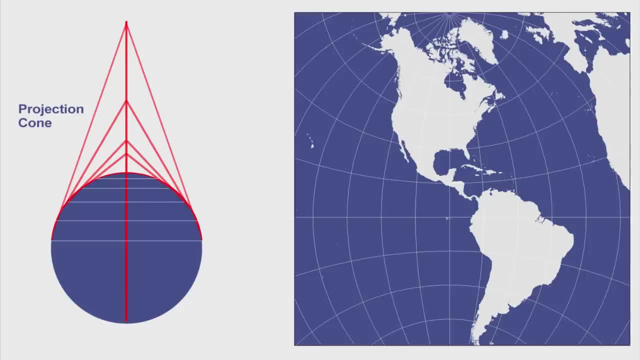 The shape of the conical map itself can be kind of strange if it's trying to show the entire world. It is worth noting that there are more types of projections than just the conical ones, And even within cylindrical there are different types of ways of doing the cylinder, and within conical there are different ways of doing the cone. 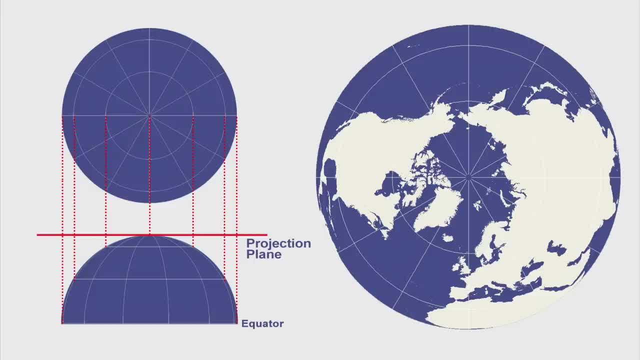 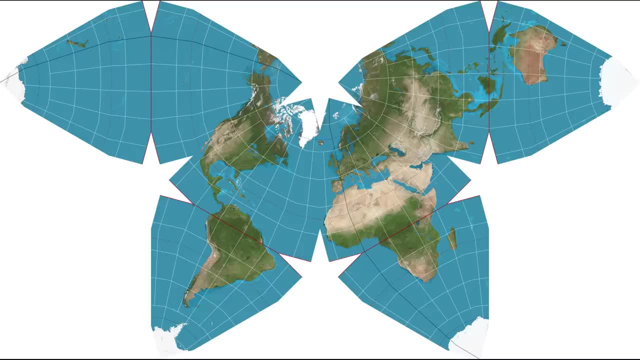 You also have planar projections which follow azimuth, as well as polyhedron type projections that do a pretty good job of preserving shape and area, but they look really weird. But for the sake of this video, I'm going to talk about primarily just cylindrical and conical. 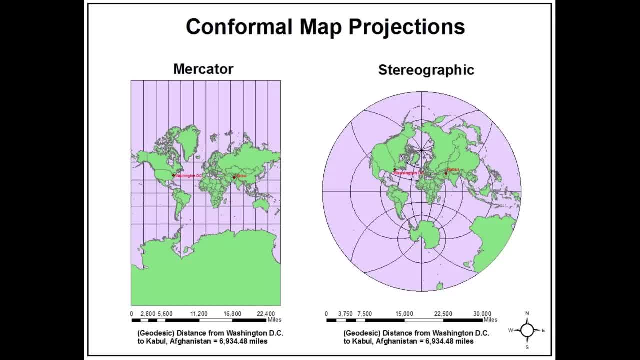 So now let's talk about some of the individual projections. First, I want to discuss conformal projections. These are ones that preserve the proper shape of what's being shown on the map at great compromise to size. So I want to start off with talking about everyone's favorite projection, the Mercator. 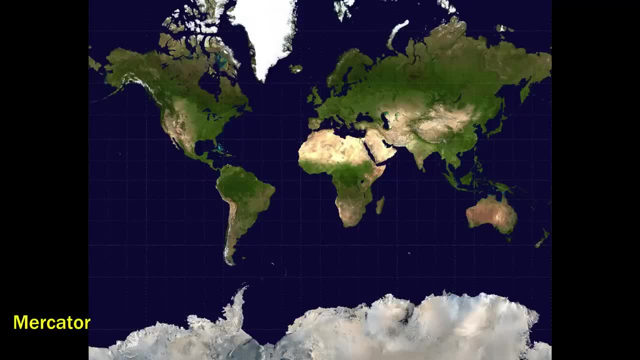 This is a very old projection, created in the mid-1500s, and it was used primarily for navigation on the seas. Some of the benefits of the Mercator is that all of the lines of latitude and longitude intersect at 90 degree angles, as well, as north is always up and south is always down. 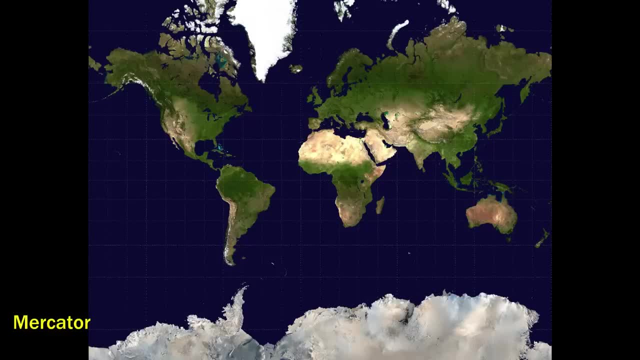 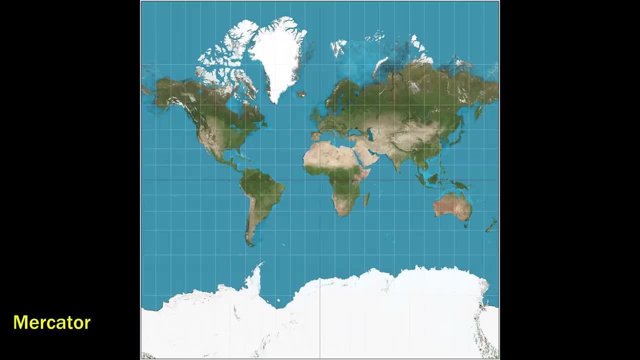 But the obvious compromise with the Mercator projection is size. The polar areas are greatly stretched out and can actually look kind of comical. It usually cuts off the most arctic and antarctic parts of the map. so if you were to see an entire Mercator projection, 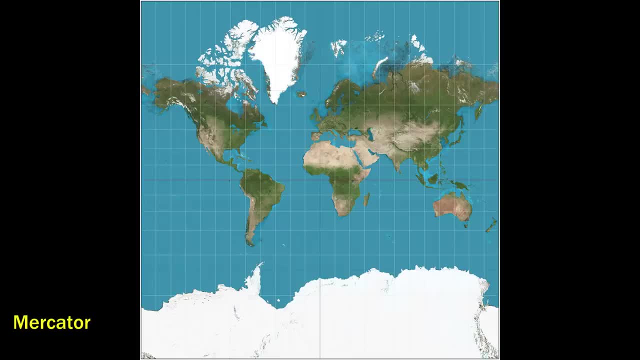 the arctic areas and antarctic areas look even more ridiculous, But as being primarily a projection used for sea navigation, there wasn't a whole lot of navigation in the arctic and antarctic areas at the time, so the mid-latitude areas are preserved pretty well. 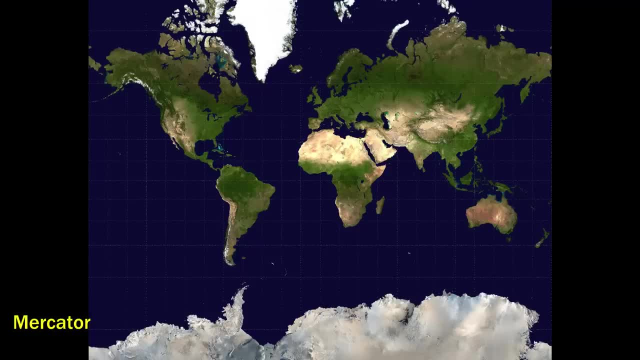 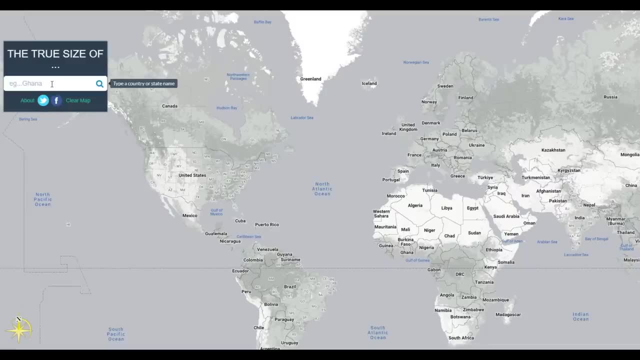 But nonetheless, the Mercator projection is responsible for why so many people think arctic areas are much larger than they really are. So I'm going to show you just how much Mercator projection distorts size by using this website. TrueSizeOf. 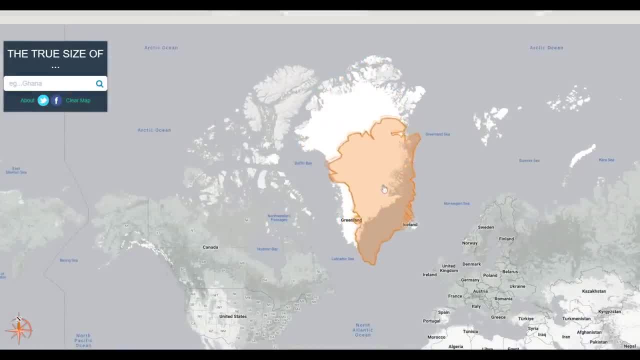 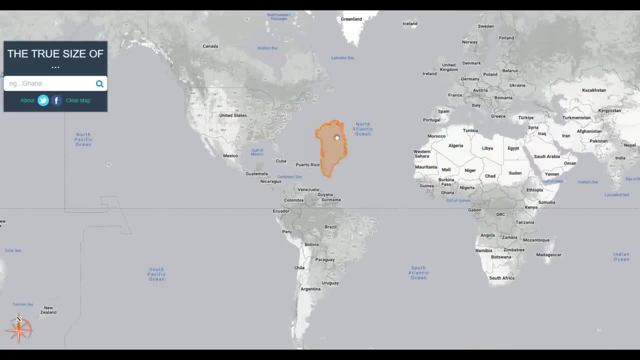 It's a great website to mess around with and I'll leave a link to it in the description So you can take a large landform from a higher latitude area like Russia or Greenland or Canada and superimpose it on an area in the mid-latitudes to see what its relative size actually is. 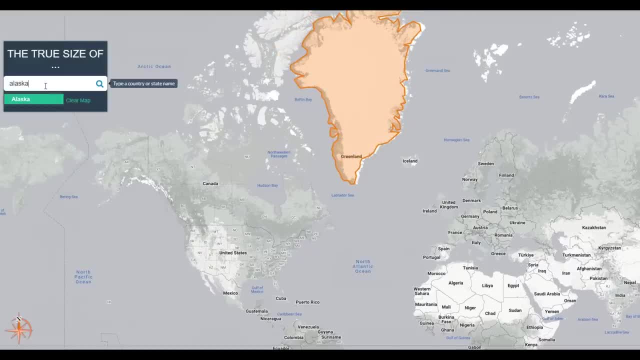 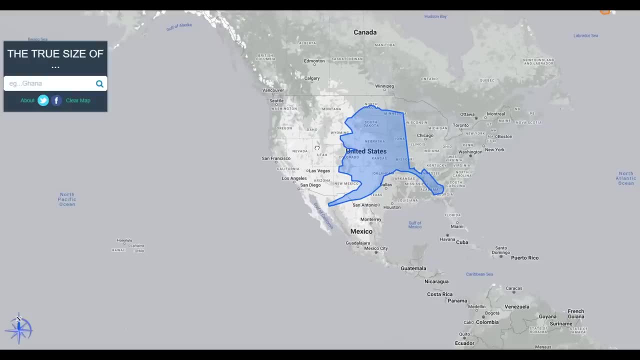 So a Mercator projection is not a great one to show the entire globe, but it is great for showing the entire globe. It doesn't show any much localized areas. Maps like this are usually not very good at the small scale, but are much better at large scale. 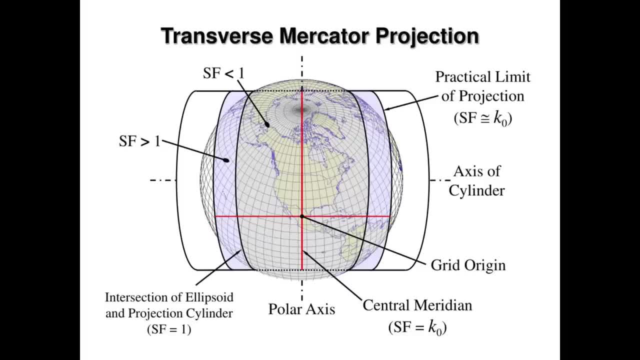 So many of the applications that we use with maps at a larger scale to show a smaller area are often shown in universal transverse Mercator, And that's just a transversely oriented Mercator projection but zoomed in to a much larger scale. 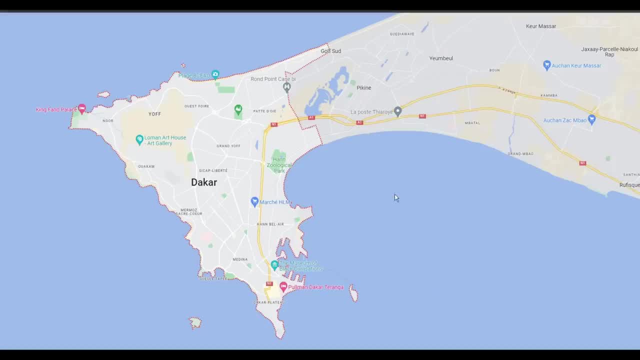 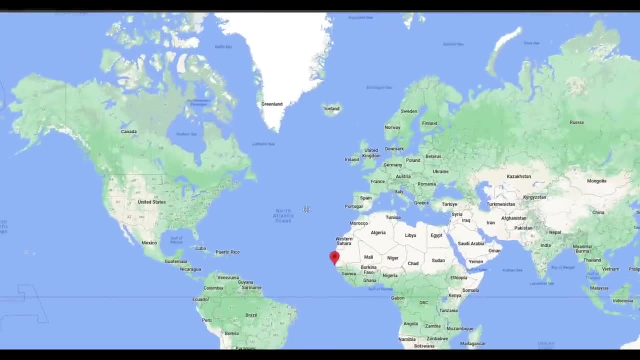 And I didn't mention this before, but a large scale map shows smaller areas. So a small scale map is used for a globe or large continental regions. A large scale map shows small areas And this is the map projection used by Google Maps and most other map services. 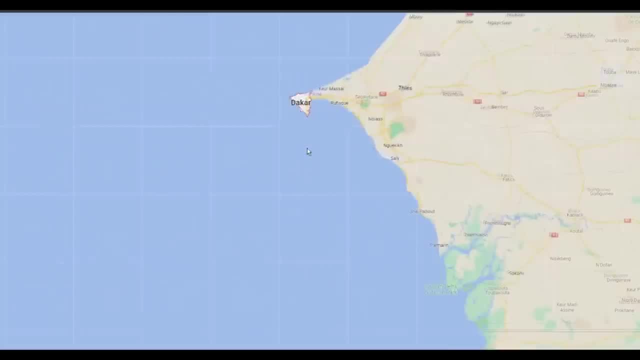 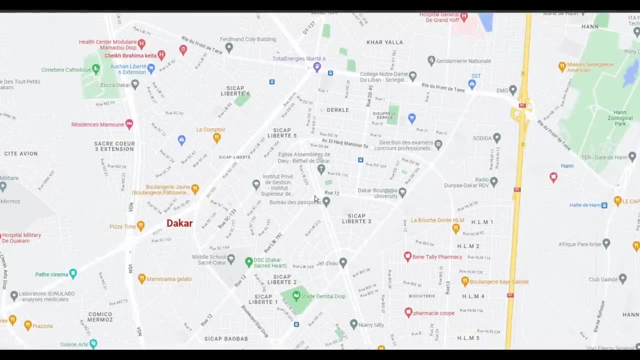 And with Mercator north is always up, south is always down, so that makes for very good local navigation directions. So the Mercator projection is by far the most well-known one of the conformal shape projections, but it isn't the only one that is conformal to shape. 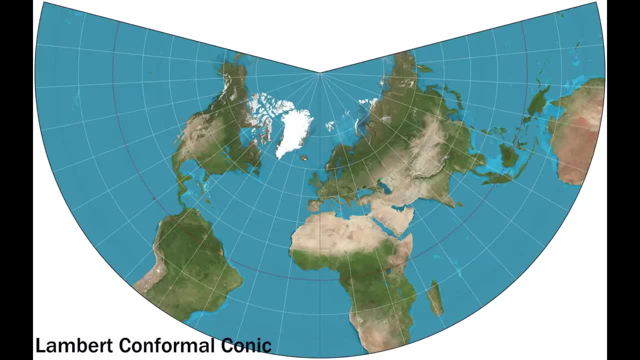 Another one in this category is the Lambert conformal conic projection. This one is often used for aviation navigation, because a straight line on a map is pretty close to a great circle on a globe, So this isn't one for most people's day-to-day use. 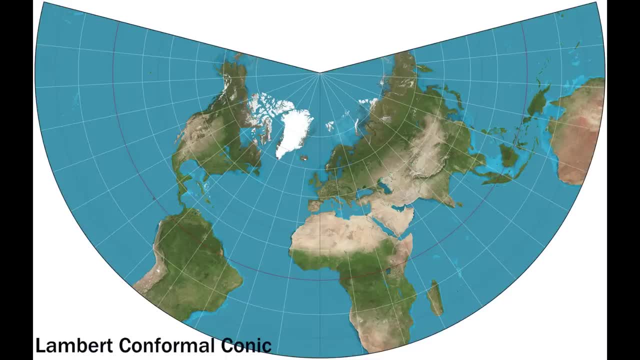 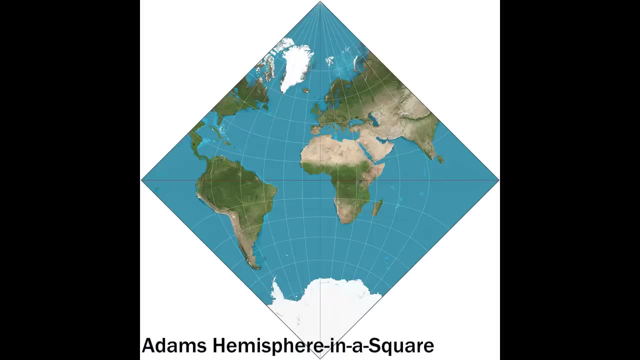 but it is an important one in terms of aviation. and again, following great circles, Here's another one that conforms to shape. It's called the Adams hemisphere in a square projection. And well, it's a hemisphere in a square. This is an example of a projection that doesn't really have any practical uses. 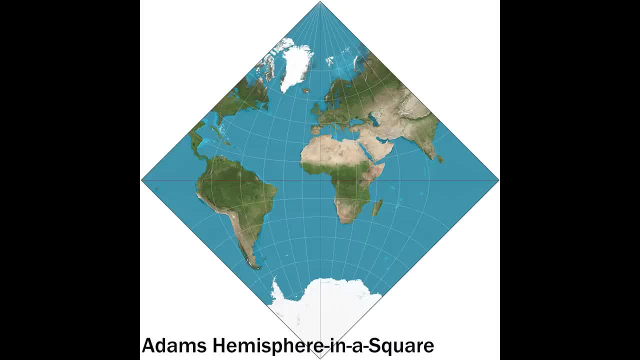 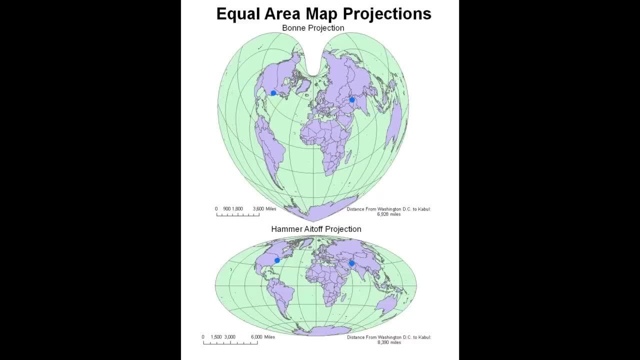 but looks kind of cool, I guess. But much like a Mercator. the areas in the polar regions are distorted and look much larger. The next type of projection I'm going to discuss are the equal area ones, As the name implies. 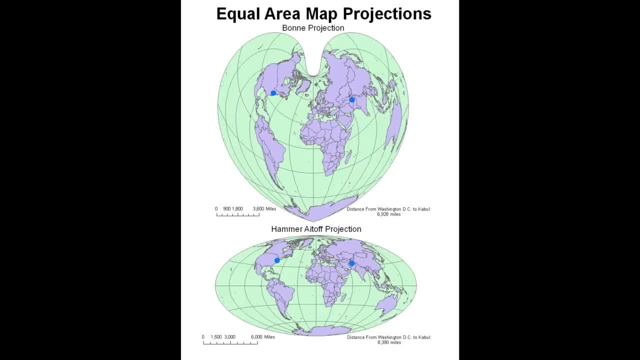 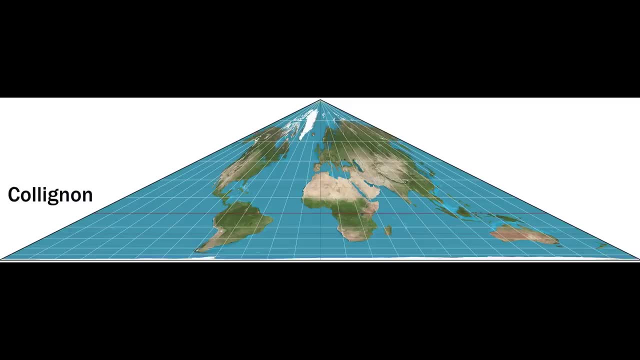 the area of things shown on a map is perfectly preserved, but scale and shape are distorted. So, to give you, one of the more extreme examples of an equal area map is the Collignon projection. So, on an equal area map, each of the landforms shown on here, 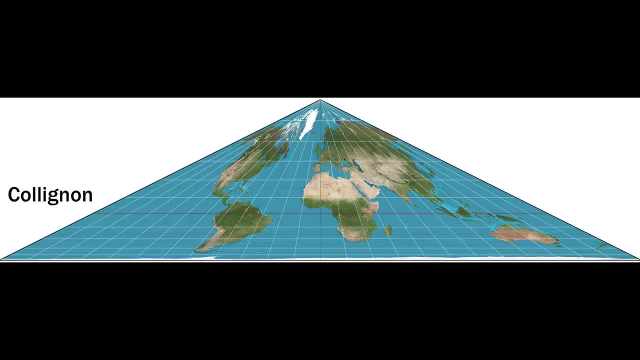 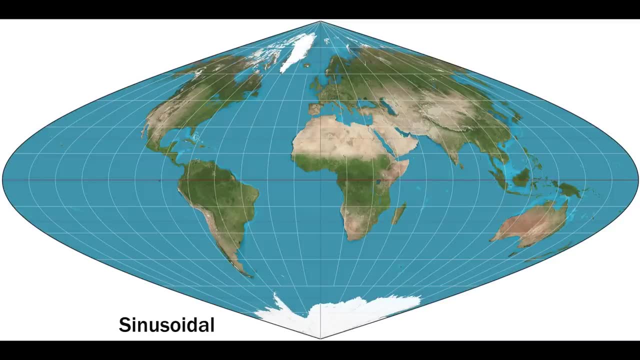 that is the proper area of it, but, as you can tell, the shapes are way off. This particular projection has uses in astrophysics, but not really much else. Another equal area projection is the sinusoidal. This looks a little bit more like a normal map. 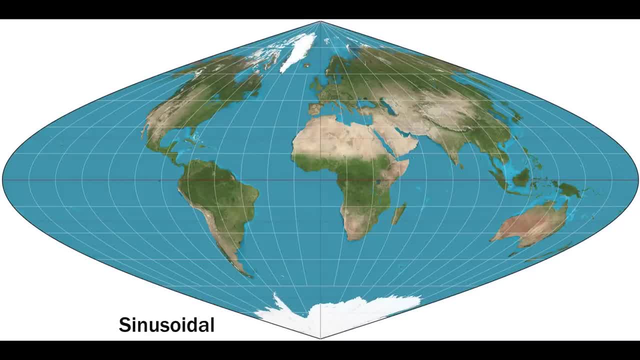 but, as you can see, it is still very distorted in terms of its shape to preserve area. But what defines this projection is the fact that the poles are points and therefore you get a more accurate representation of the size of the polar regions in relation to the rest of the Earth. 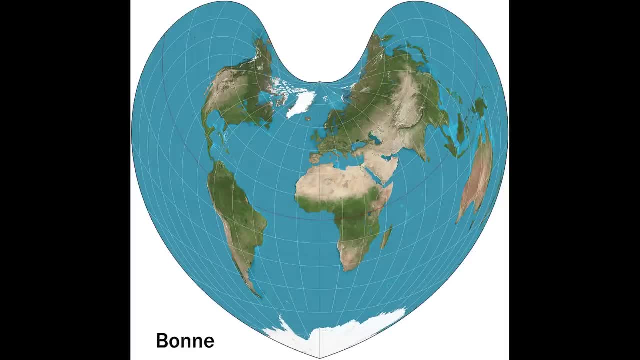 The bond projection is one of many that has kind of a heart shape to it. So for this bond projection it looks kind of strange at the global scale but it is used quite often at a more large scale to show smaller local areas. Another one of the heart-shaped projections. 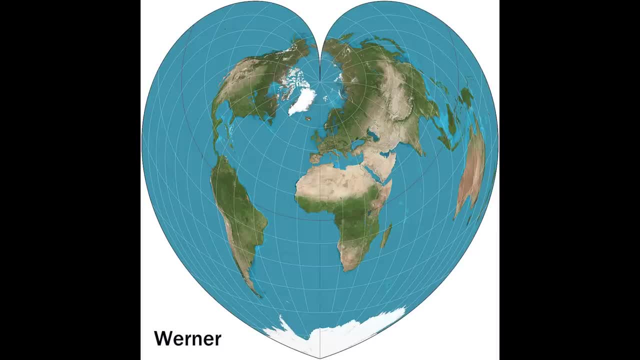 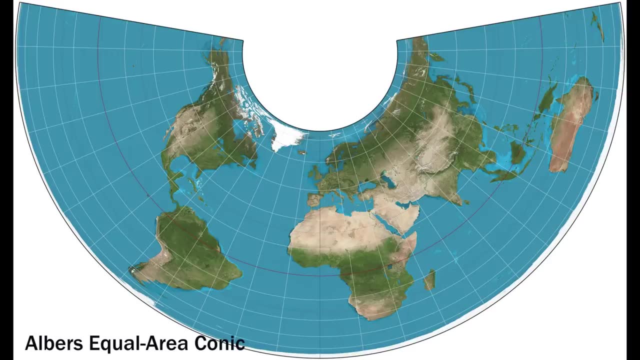 is the Werner projection And again, these heart-shaped projections are often used at the larger scale to show more localized areas. One that many of you might be quite familiar with is the Albers projection, For example, if you're familiar with the US Geological Survey, topo quads. 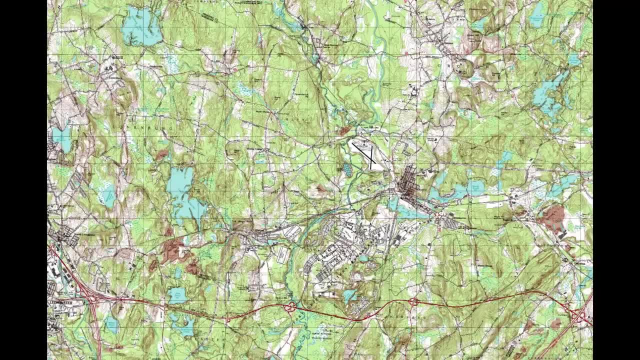 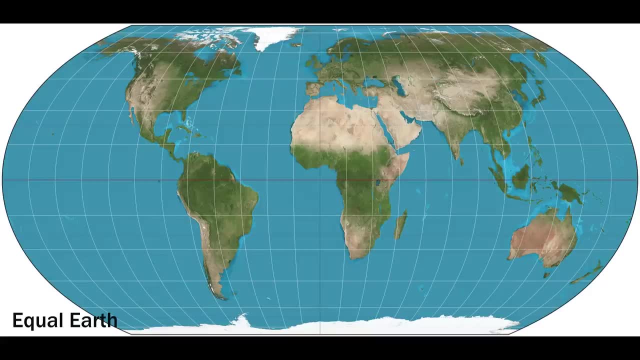 they use the Albers projection on those, And this is also the projection that the US Census Bureau uses for mapping. One of the most recent projections to be created is the Equal Earth projection, And you very well may have seen this projection used. 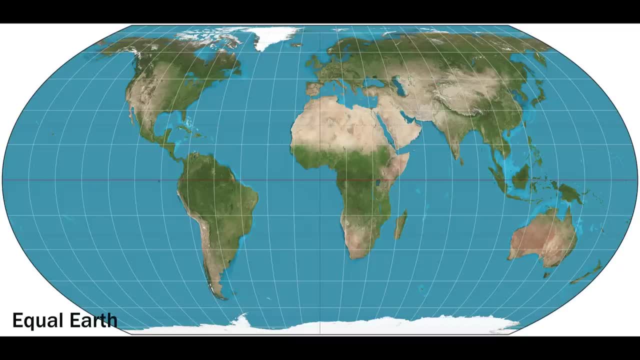 This has been adopted by many agencies worldwide. In terms of global projections, I always preferred the ones that have the curved sides, like this one or the Robinson projection that I will discuss later on. The next Equal Area one I want to discuss is the Gall-Peters projection. 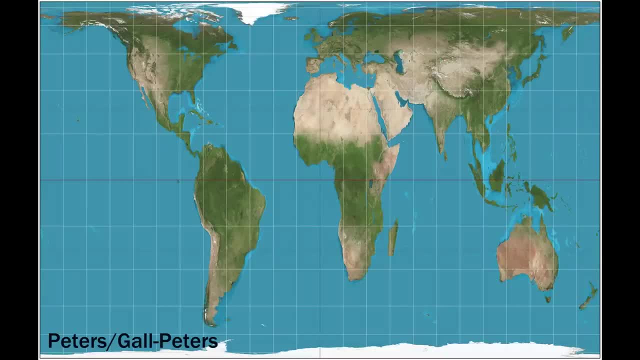 This one is sometimes referred to as the Anti-Mercator, because the Mercator stretches out the polar areas to a great extent, and this projection stretches out the tropical areas to a great extent. So, as with all Equal Area projections, there has to be a big compromise. 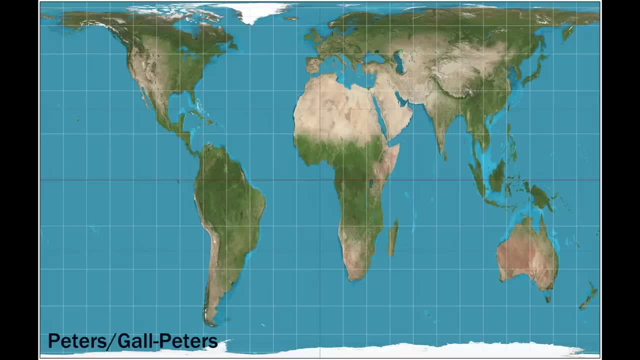 in terms of shape. Many people think that this projection was created recently to kind of offset the Mercator. However, it was created in 1885, so this goes back quite a ways. So you'll sometimes hear some debate over which one's better- the Mercator, 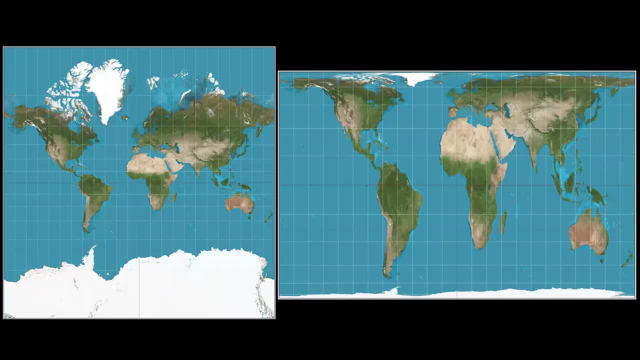 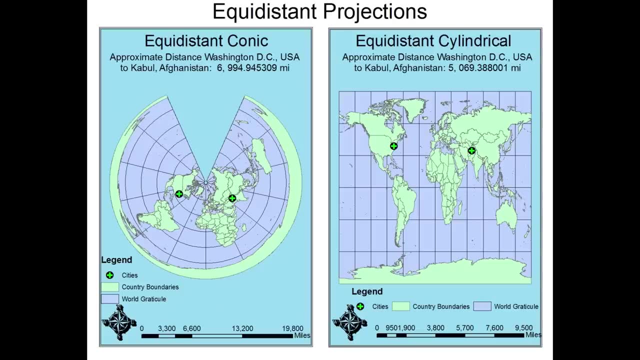 or the Gall-Peters. Can we just say they both suck. The third major type of projection I want to discuss are equidistant ones And, as it sounds, it preserves the distance from one point to all other points on a globe. The equidistant conic projection is one of these. 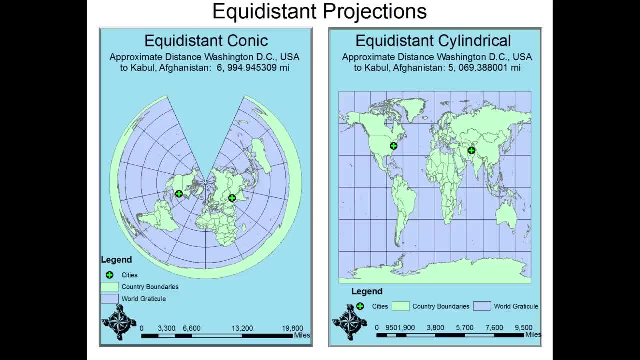 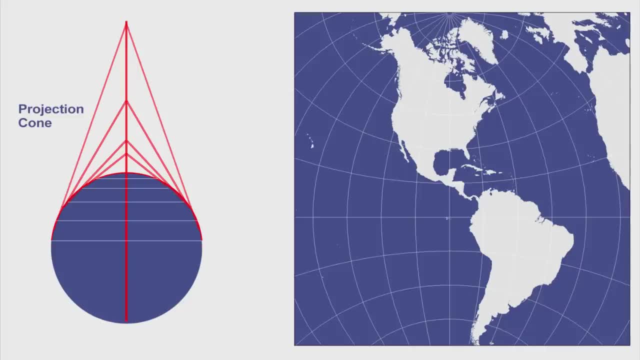 It is very lightly used, but is normally just used for small countries, showing large-scale small areas And, just like all conic projections, it's much better to show things that are oriented east-west as opposed to north-south. So a great map for Tennessee. 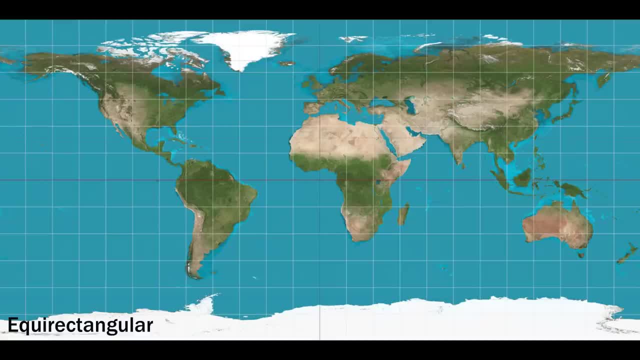 not so much for Chile. Another one that is equidistant is called the equirectangular projection And, as the name implies, every rectangle on the map is equal sized. It has some of the properties of a Mercator, but does not have conformal shape. 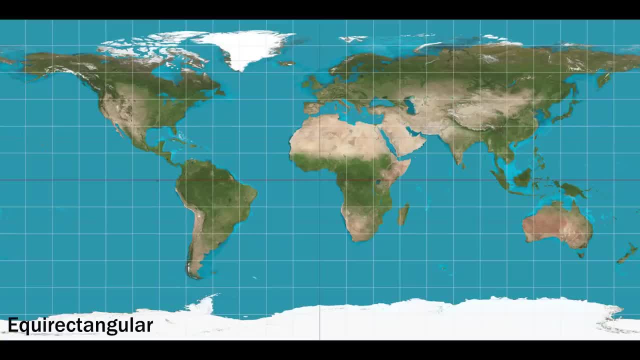 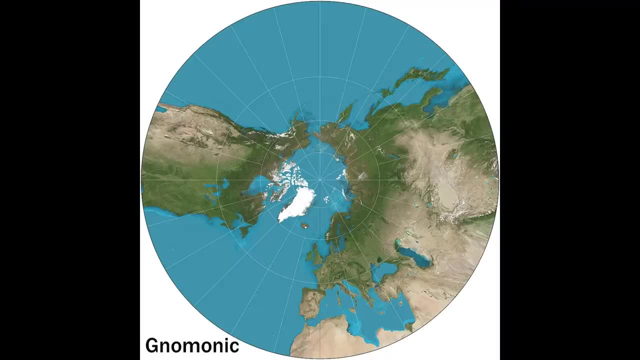 and is also not equal area. So, as a result, it doesn't really have any practical uses and is often just used for thematic reasons. Another type of projection is a mnemonic projection. The primary feature of this projection is that all great circles on the map are displayed as straight lines. 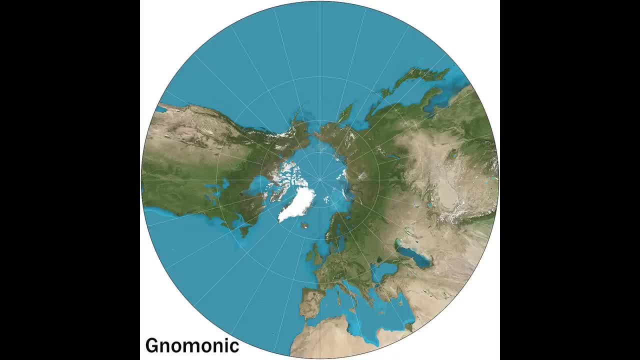 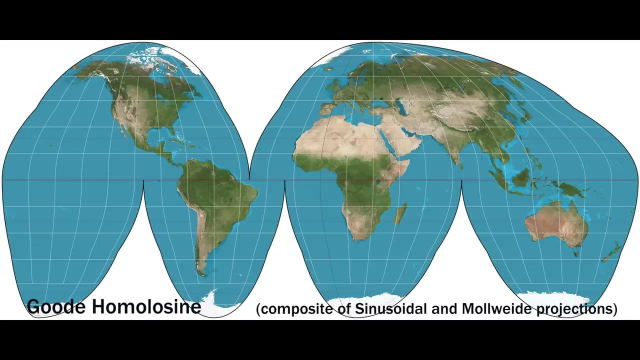 And, as a result, a straight line on this map is the shortest distance between two points. Some map projections can actually be composite projections, where it's a combination of two other ones. The best example of this is the good Hamala sign projection. When you see a map presented like this, 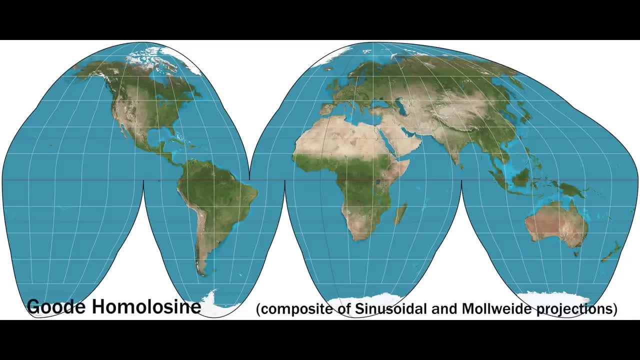 it's referred to as interrupted, And sometimes you'll hear about a projection like this referred to as an orange peel projection. So the benefits of this one is a lack of distortion in terms of shape, size or distance, With the obvious compromise here being 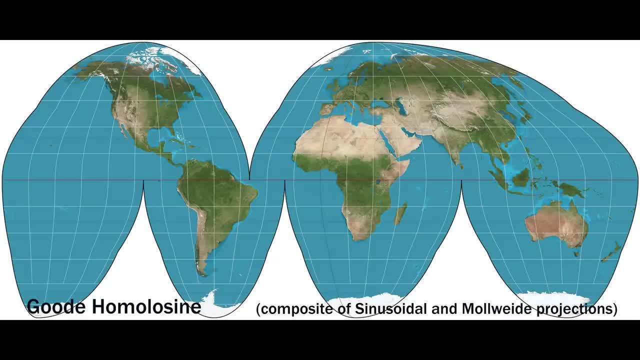 aesthetics and the map being interrupted. This is an equal area map, so each of the landforms shown on here is a compromise And because of the interrupted nature of it, the shape of the landforms is less distorted than some others. And the last general type of map projection: 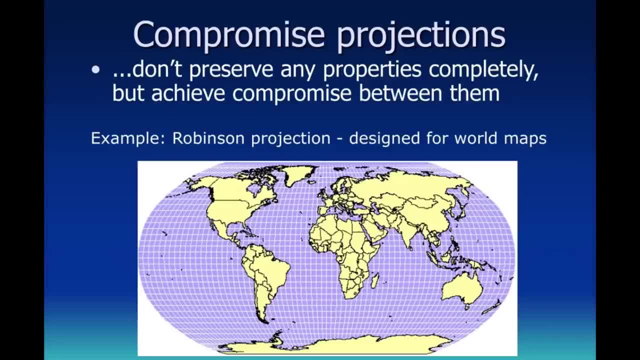 I want to discuss are the compromise ones. These are ones that do not preserve any dimensions, so they're not equal area, conformal shape or equidistant. The idea is to compromise each of the dimensions a little bit to get a more well-rounded map. 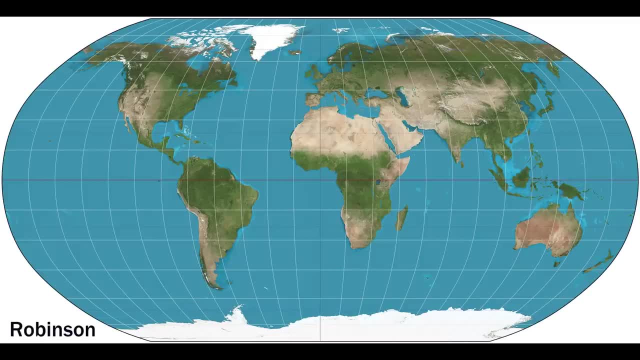 Perhaps the most well-known of the compromise projections is the Robinson, And so there are many benefits of this and some of the sides, meaning the polar areas, are not stretched out as much, But there is still some distortion, as you have to compromise a little bit of everything. 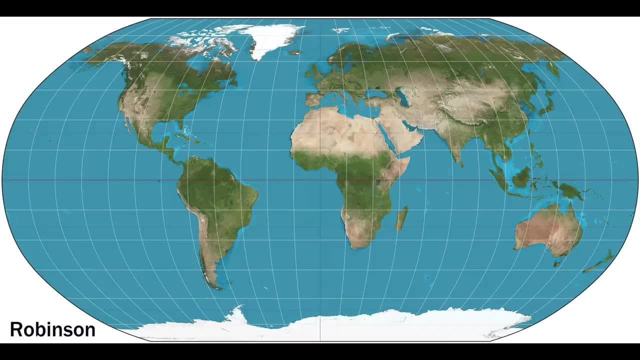 For a while this was the standard map projection of the National Geographic Society And I've always felt that the Robinson and the ones very similar to it are the overall best looking maps showing the globe. Another popular projection in the same general vein as the Robinson. 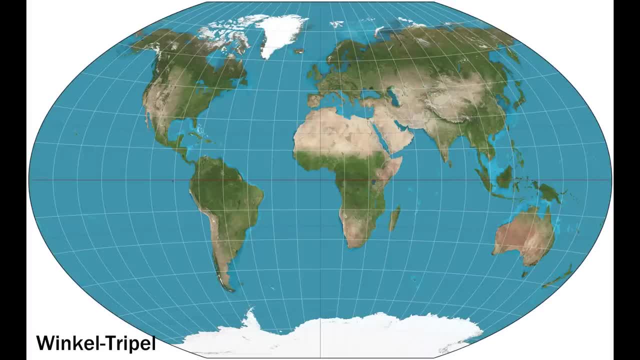 is the Winkle Triple. So lots of math to get this projection And in 1998 the National Geographic Society switched to using Robinson as their official projection to the Winkle Triple. But not all compromise maps are aesthetically pleasing. One is the: 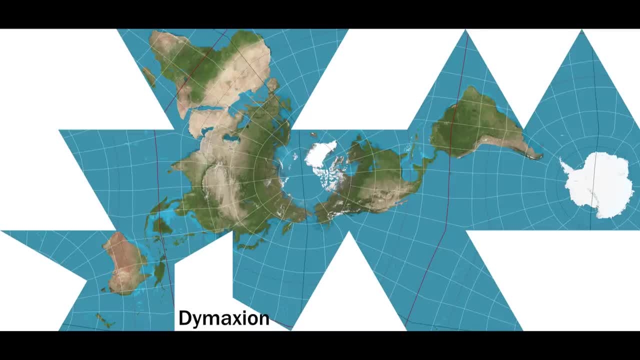 Buckminster Fuller Dymaxion map. So obviously when you see this you're thinking: what on earth literally is this? And even though this map is neither equal area nor conformal shape, it does compromise those two very little, But of course, the big compromises. 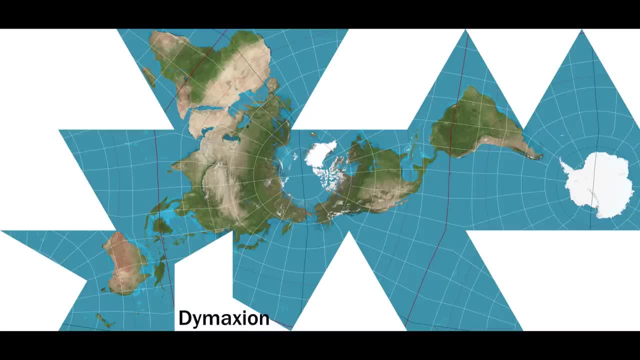 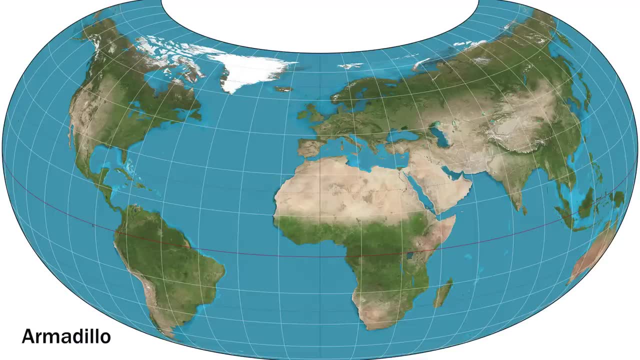 are distance and appearance. One of the more interesting compromise projections is called the Armadillo, So, as you can see, it shows about the entire course of the globe and has almost a 3D feel to it. So, more than most other projections, this shows the near spherical shape of the earth. 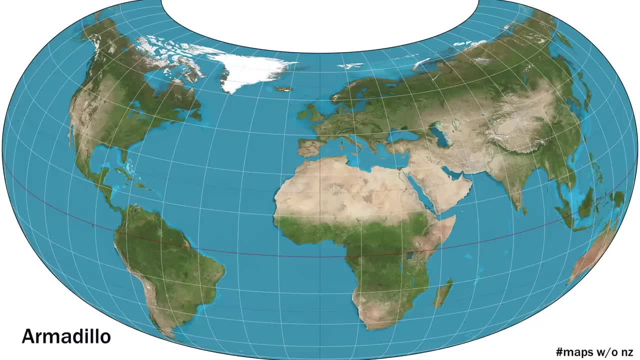 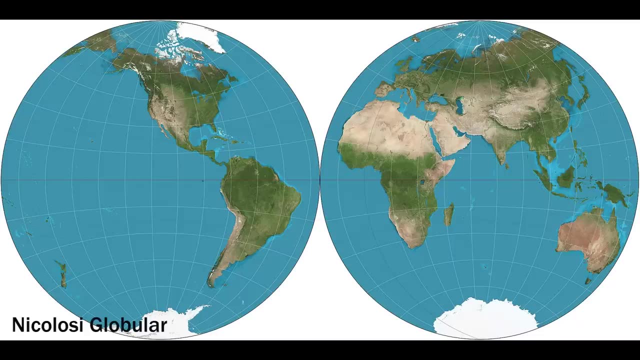 And one nice thing about this projection is that it doesn't leave anything off the map. And the last individual projection I wanted to show is the Nicolosi Globular projection. This is referred to as a polyconic projection. Multiple cones are placed on the globe. 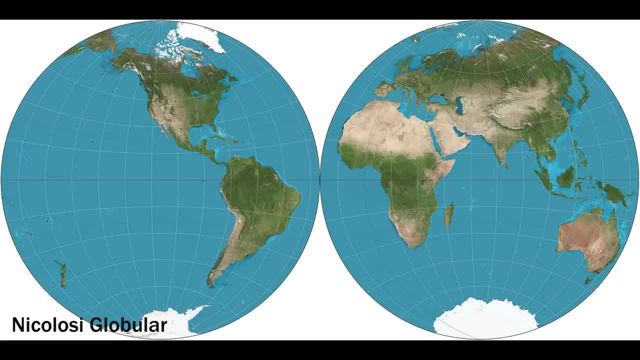 But this projection can only show one hemisphere at a time, so when it shows the entire globe it's usually like this kind of like a pair of glasses. It doesn't have a hard practical use, but it is very aesthetically pleasing. It's hard to say which of these projections 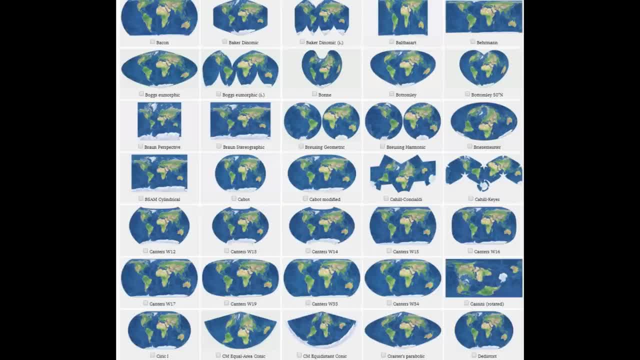 are the best and worst, because many of them have a very specific use. Others are meant to be a little more artistic or are meant to look weird, But in terms of just general use of a map, like doing a Google image search trying to find a map of the globe- 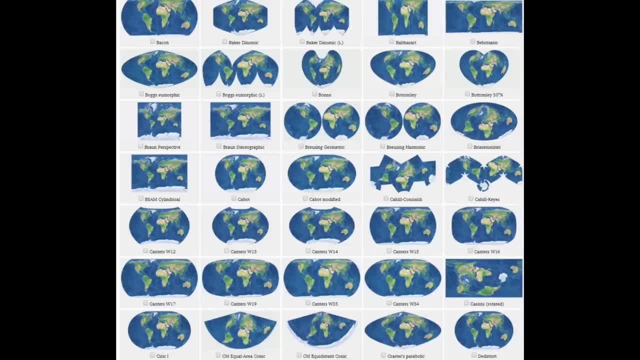 that shows whatever. I like to think we'd get away from using the Mercator and Galpeter style perfectly rectangular maps and move more towards the Robinson and Winkle equal earth style maps that have the rounded sides. I think those are just much better. 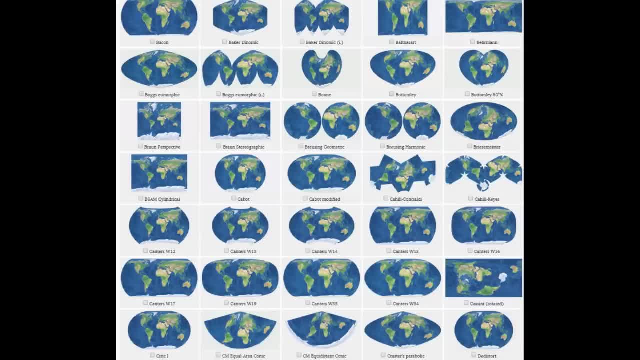 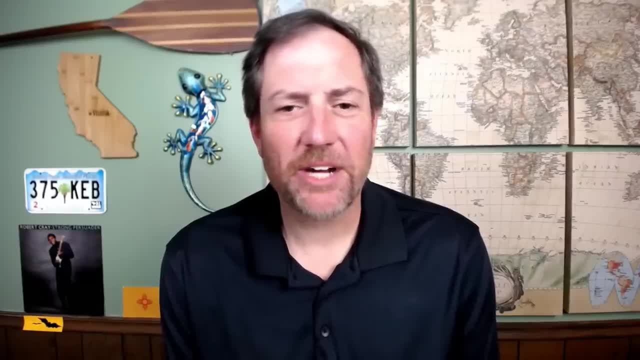 in terms of the overall aesthetic appearance, but also gives a more accurate representation of what you're actually seeing on the earth. I hope you enjoyed this video. If you did, please give me a thumbs up to let me know you approve and subscribe to this channel. 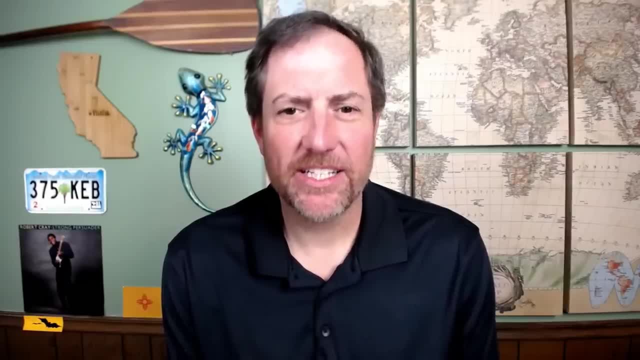 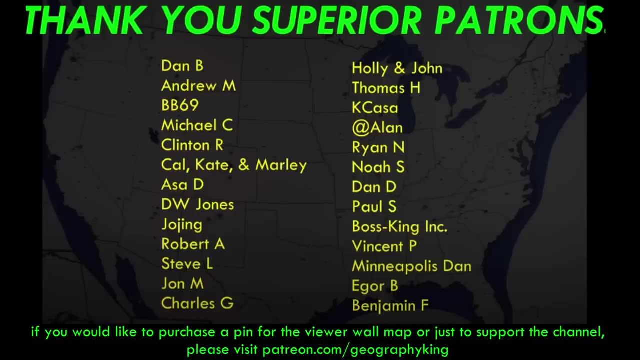 if you're interested in learning more about geography from a nerdy perspective. But yeah, thanks for watching Geography King signing out. I want to give a special thanks to my superior patrons for their support. If you'd like to support a wall map. 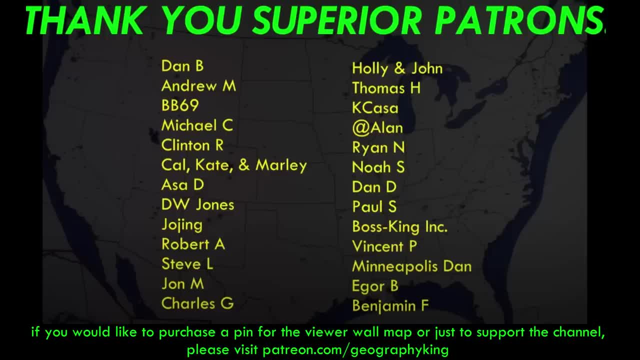 or just to support the channel. check out my Patreon page Link in the description. And, as always, thank you very much.